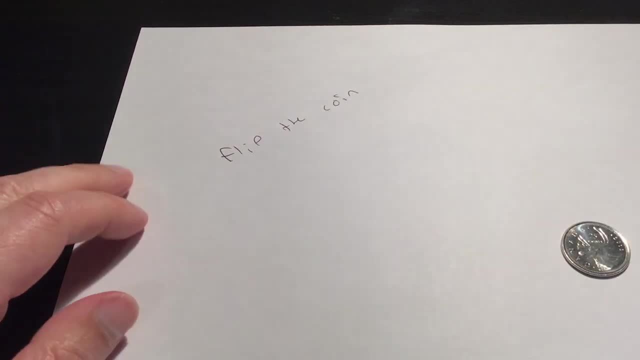 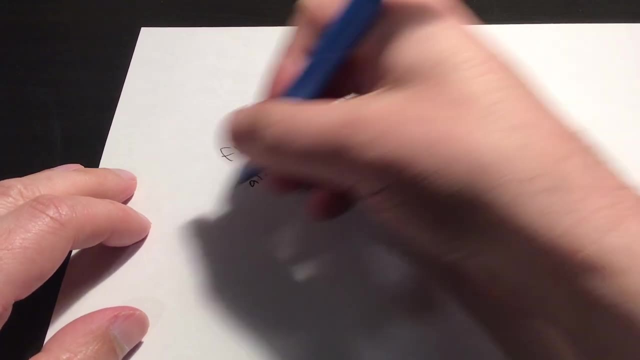 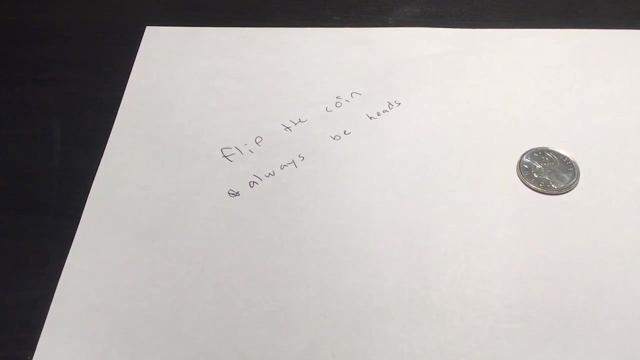 I mean, there's not a whole lot else you can do, And I think it will always be heads. That is my prediction. Do you think it's a good one? Let's find out. So that's my suggestion. Or maybe I'll say this: 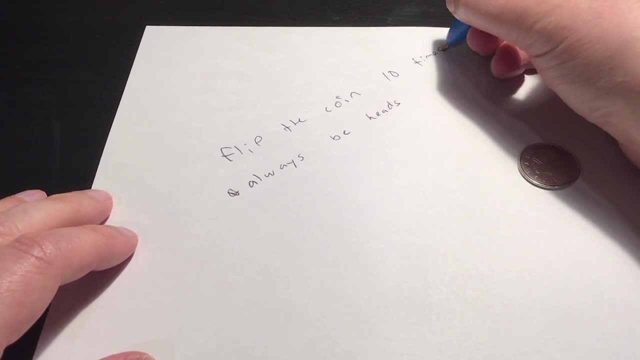 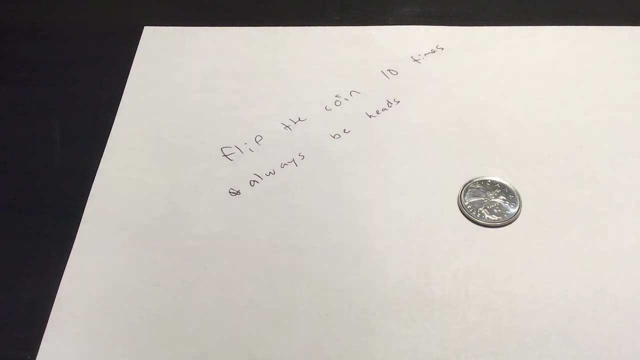 I think I'm going to flip the coin 10 times and it will always be heads. Here we go. I don't know if I can do this while looking at the video. Oh, I can't. Well, let's count that one. Hey tails. Okay. so now I need some way to keep track. So there's. 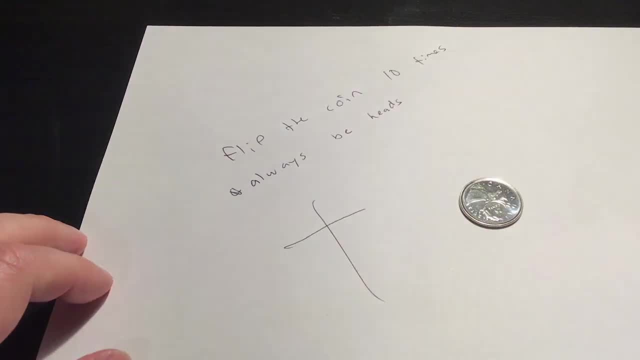 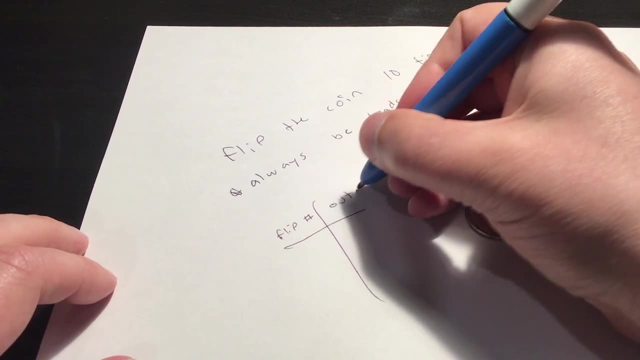 you know lots of ways, Since I'm doing it 10 times. I think sort of the easiest way is the old T-chart baby. So I'm going to go flip number and let's say outcome. I could have wrote heads or tails, whatever. So flip one, two, three, four, five, You know. 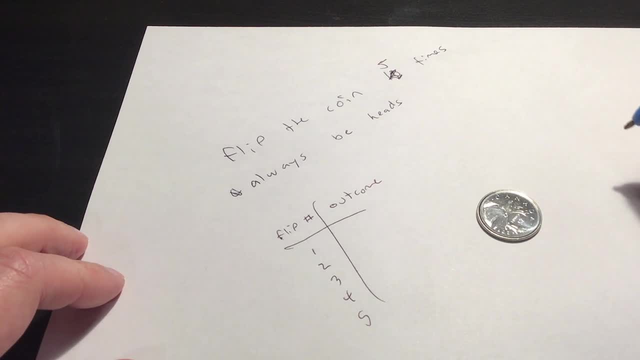 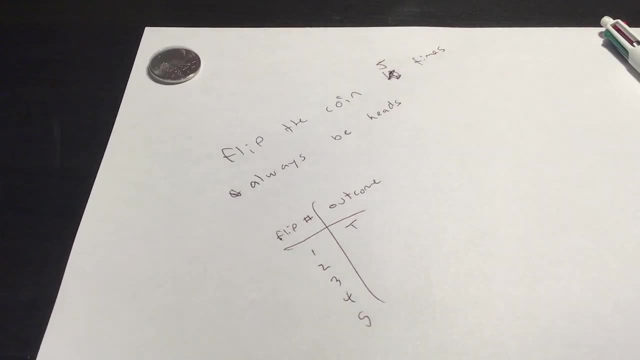 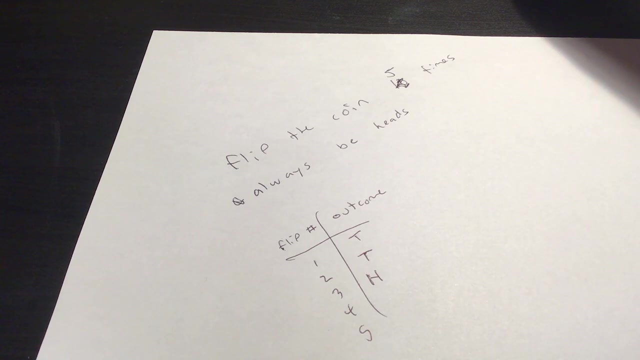 let's make this five. just for the sake of the video, Make it a little shorter here. So, number one: what do we get? Tails, Okay. second flip: Tails. So far, my prediction was awful: Heads, And it's off screen, but it is heads. Okay, and one more flip. 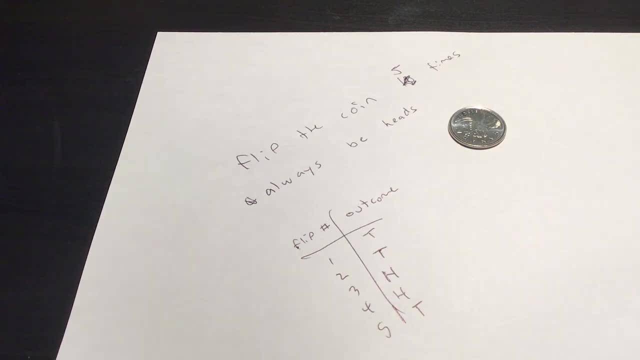 Tails. All right, so there's my experiment. My prediction was that it was always heads. it was a terrible prediction And I don't really have any reason right. I didn't say why. I didn't say I think it always be heads because, and then some reason right. And then I actually conducted. 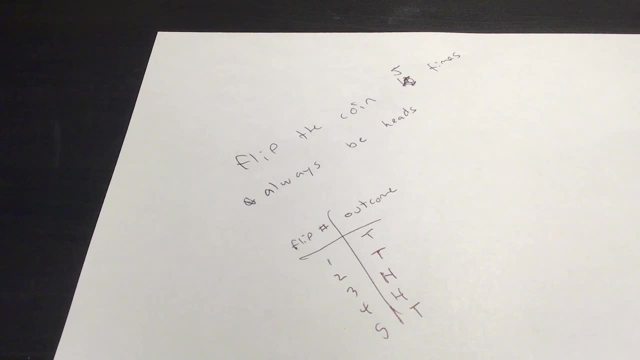 my experiment with five flips. I got tails, tails, heads, heads, tails. Okay, so there you go, All right, why was my prediction bad? Well, it didn't really make any sense. A better prediction would have been three and two right, Or if I'd kept it as 10 times. 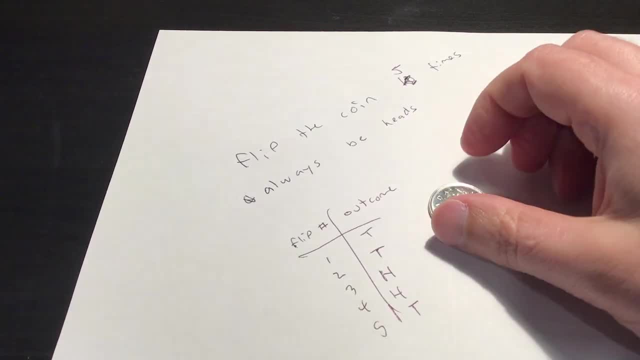 I could have said I think it's going to be even, Because the thing with the coin is that it's it's a fair flip, right? I mean, you got, you got tails, you got heads. there's only two. 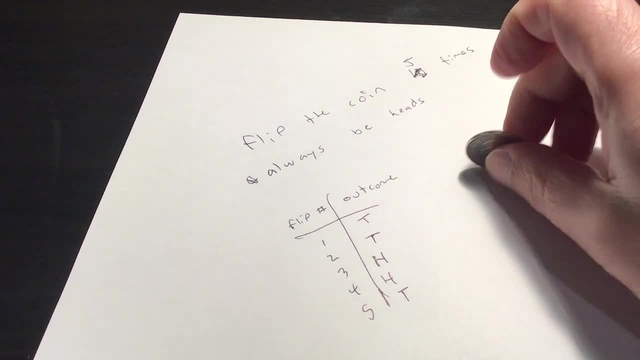 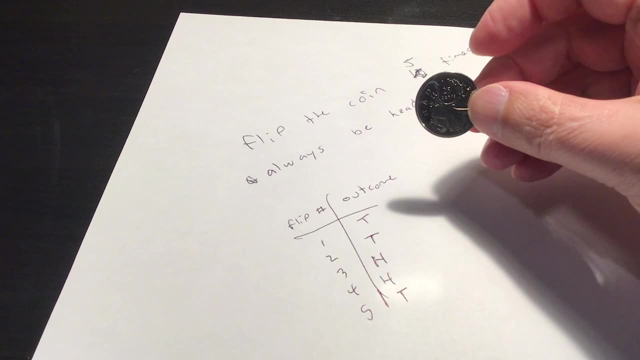 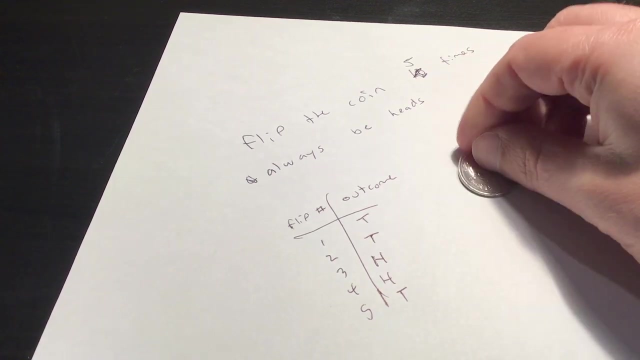 choices. It's never going to land, sort of, on its side. it's always going to land on one side or the other. You know, you could get like really annoying and say I actually scraped off the metal off the coin And I discovered that the tail side actually has slightly more, which means it's a little 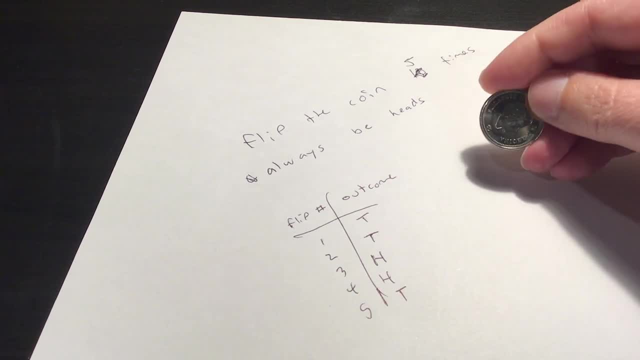 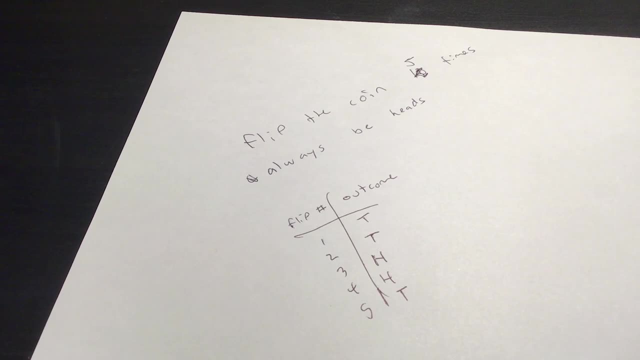 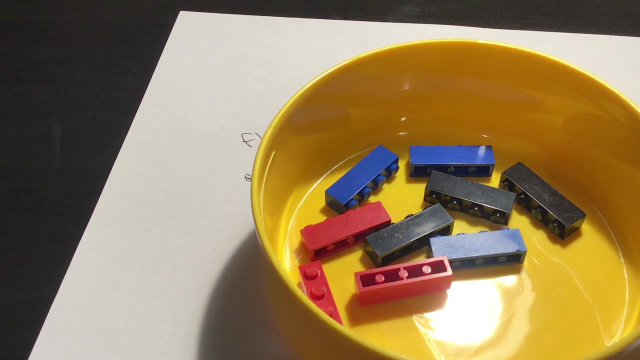 heavier. So heads, okay. whatever You know, it's generally thought of as being a fair share. Okay, So there we go. Let's do a second experiment. now We're going to use this. So I got my. I got three of each color. I've got three black Lego pieces, three red, three blue. 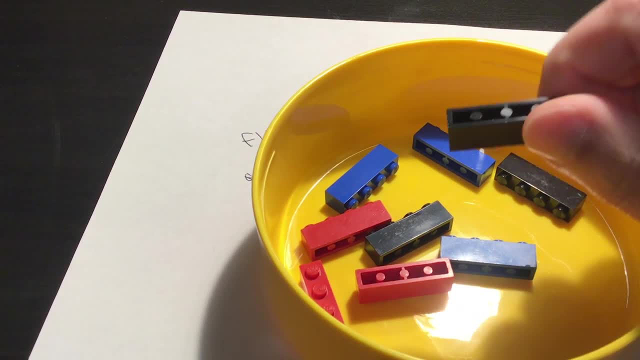 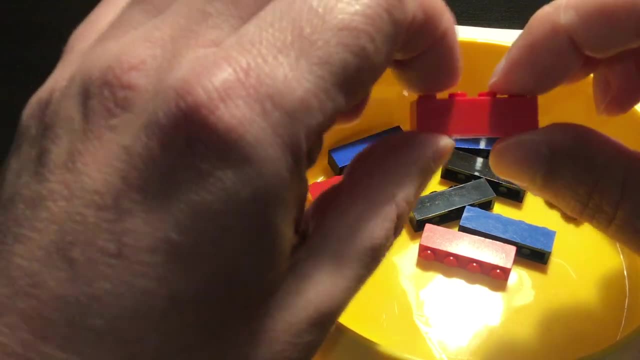 and they are all the same. Okay, that's important If I was all of a sudden using different ones, like if I said, okay, I've got you know, I'm going to use Lego pieces that are four bricks long by one brick high And I'm going to use three red, three black and three blue. It's a fair. 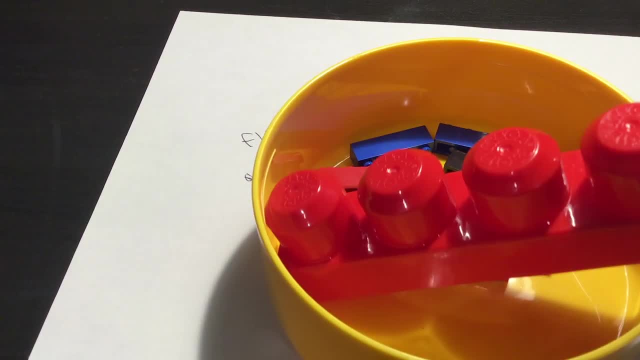 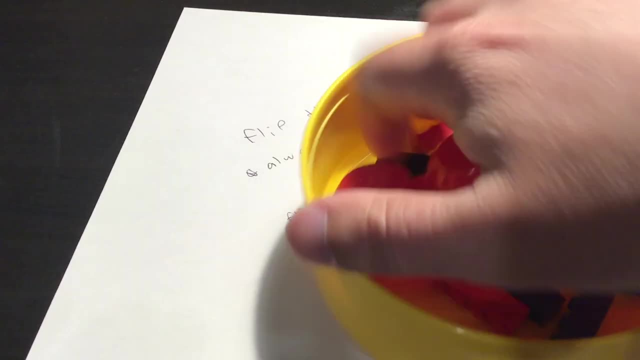 experiment right. If all of a sudden I swapped one of these reds out for that one, then all of a sudden the experiment's no longer fair right? Because if I reach in and close my eyes, oh, I picked red. I wonder what I'll pick next time. Reach in and close, Oh. 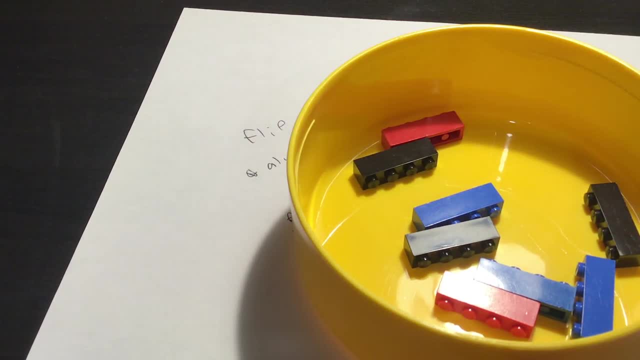 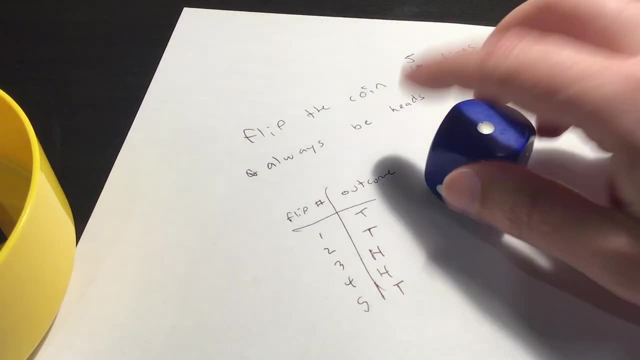 I picked red again. right, It's no longer a fair experiment. So for this to be a fair experiment, it needs to be a fair setup. right, Every piece needs to be the same size, just like with a dice. right, All the sides are the same. If it wouldn't be a fair experiment if, all of a sudden, you had 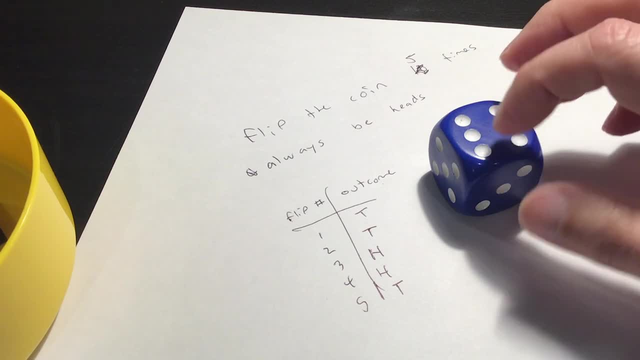 you know, one, two, three, four, five and then a second five on the dice. you didn't have all the, you didn't have the six right. It wouldn't be a fair experiment. Okay, Same with if you decided to. 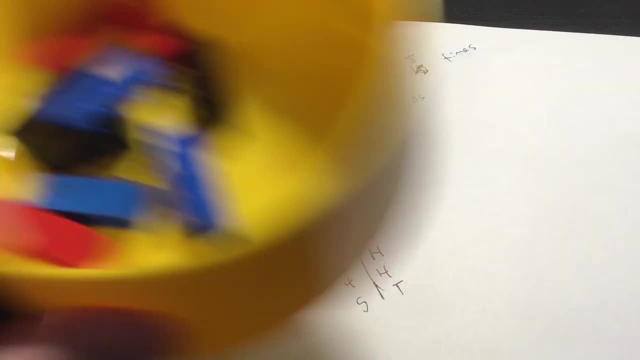 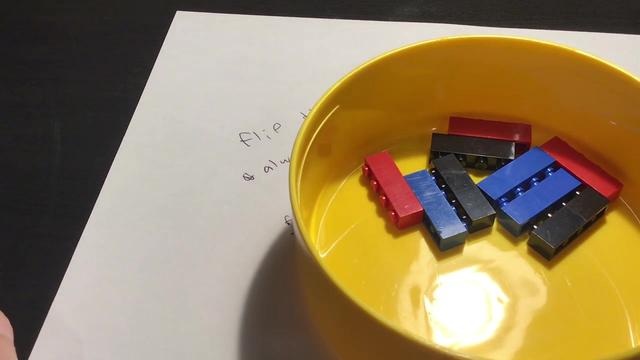 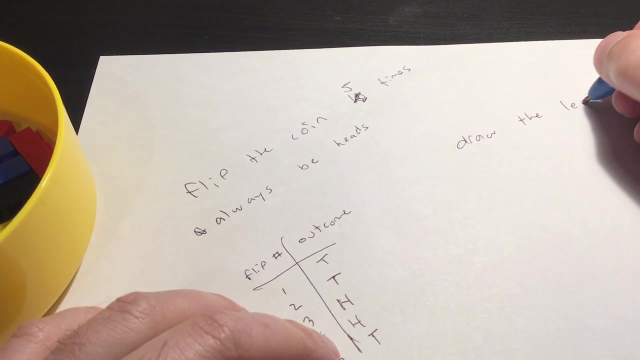 use a, a coin that had heads on both sides, right. So that's the idea behind a fair experiment. Okay, So I have nine total pieces in here, um, three of each color. Okay, So my experiment is going to be called: uh, draw the Lego piece, And by draw I mean pick out, not draw, Don't worry. 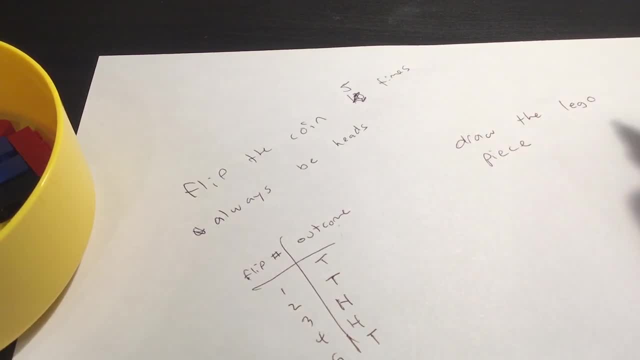 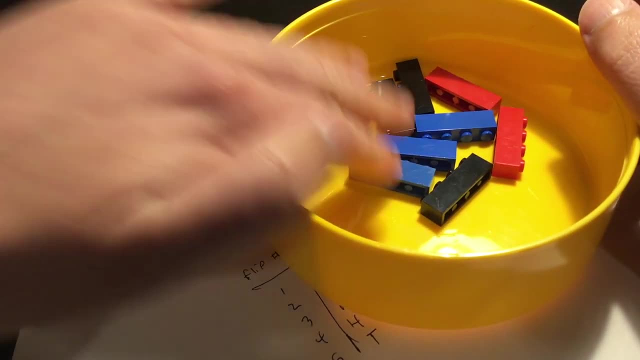 You see my handwriting. Um, you, we don't want me. Yeah, you know. Okay, So draw the Lego piece. So my prediction is: this time I'll do a real prediction. So I predict that. how many draws should I do? Let's say nine. Hey, there's nine. 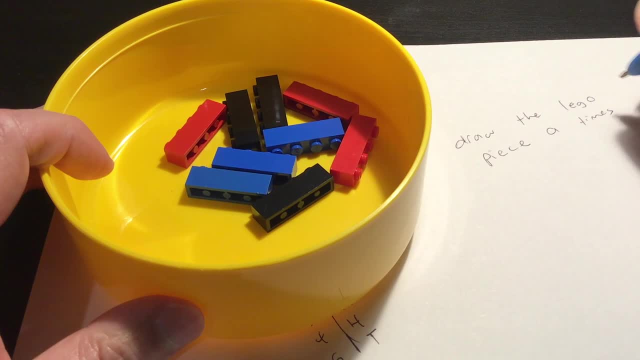 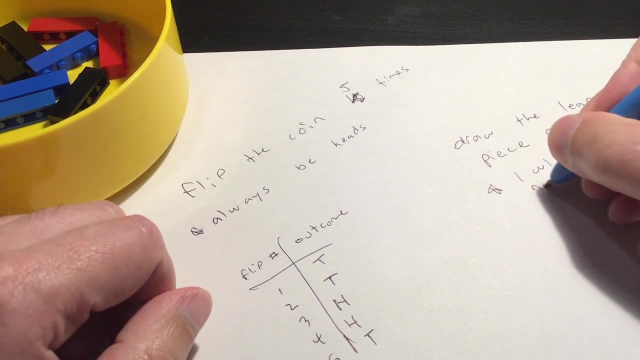 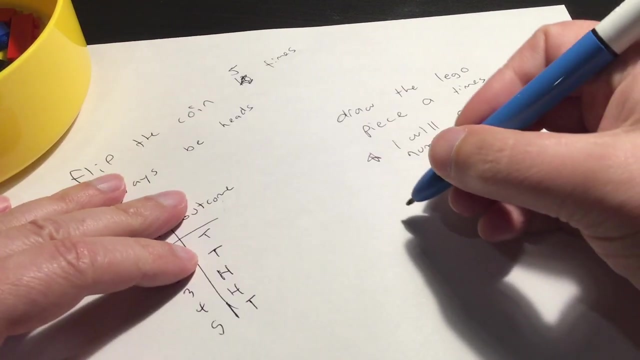 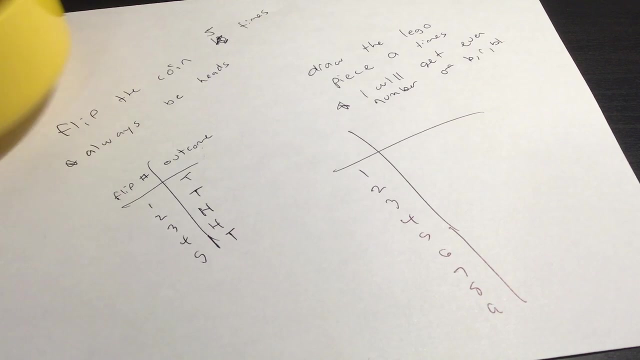 pieces. So draw the Lego piece nine times And I predict that I will get even number of blue, red, black. Okay, So nine draws one, two, three, four, five, six, seven, eight, nine, 10.. Okay, And here we go, And I am going to close my eyes. And here we go. First draw black. 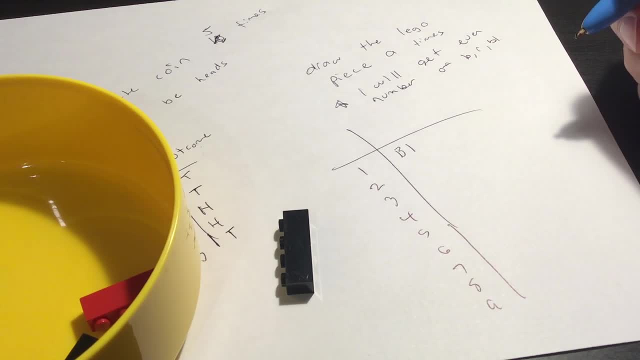 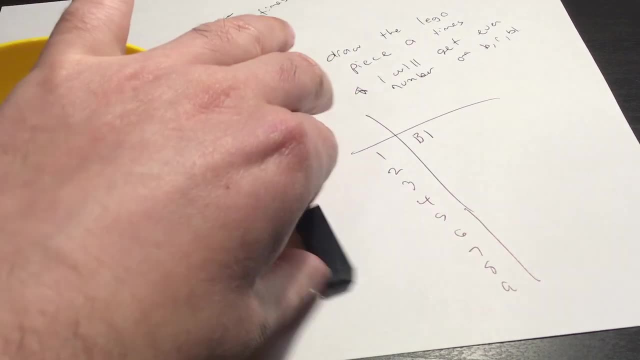 I'll do BL for that. Now you kind of have to decide what you're going to do. Are you going to replace the piece each time, Or are you going to not replace? I'm going to replace, And I'll tell you why I'm replacing, because I feel like it's like it's like rolling the dice When I roll. 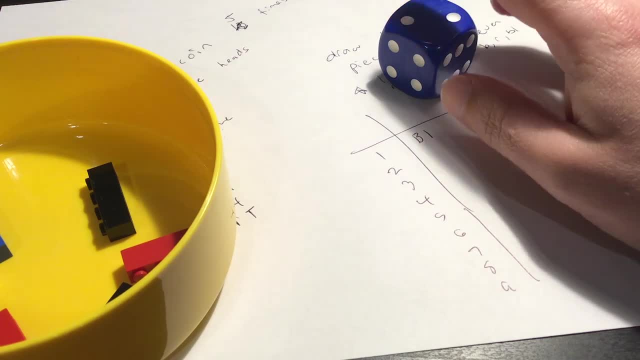 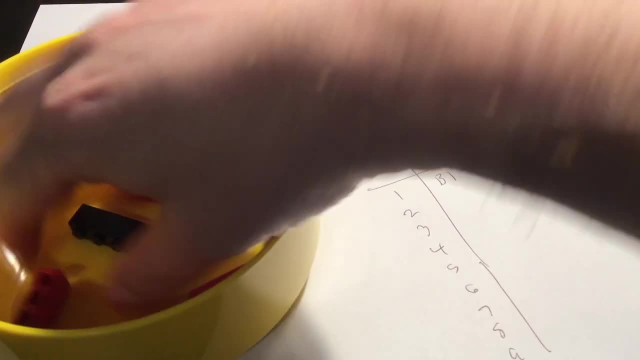 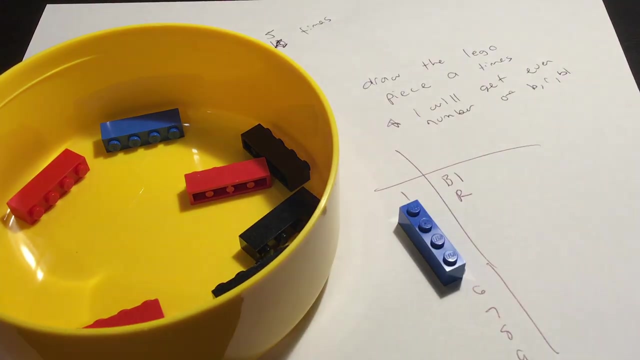 a two, I don't then take off the two and it's no longer an option. Okay, But you need to kind of think about that before you do the experiment, before you do your prediction. Okay, Eyes closed. Second: draw red. Okay, Throw it back in. Hey, so far it has been. 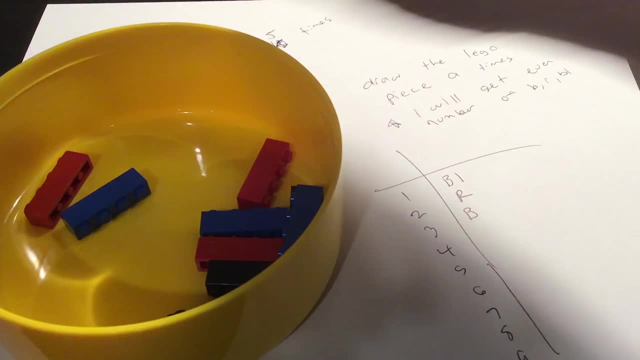 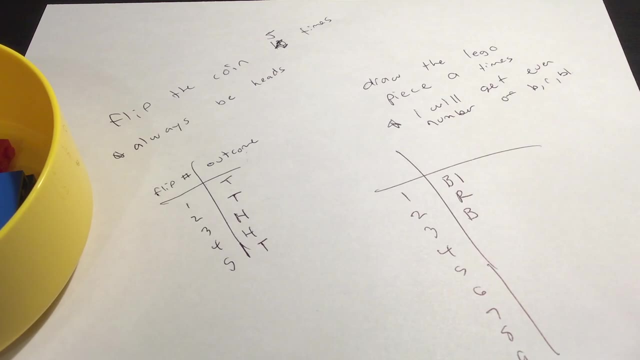 even. Okay, I would keep going. I'm not going to do this for the whole video, but we got kind of lucky that it turned out even Now. here's the thing It may not right. It's very, very likely. 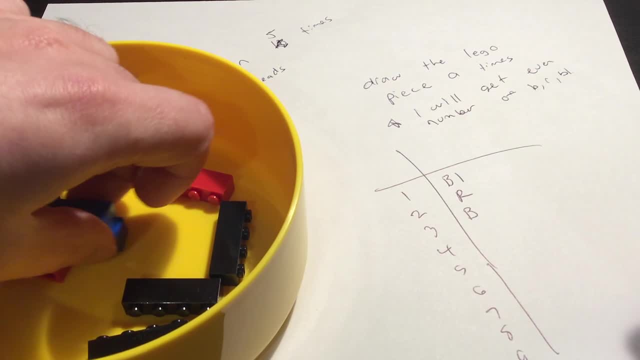 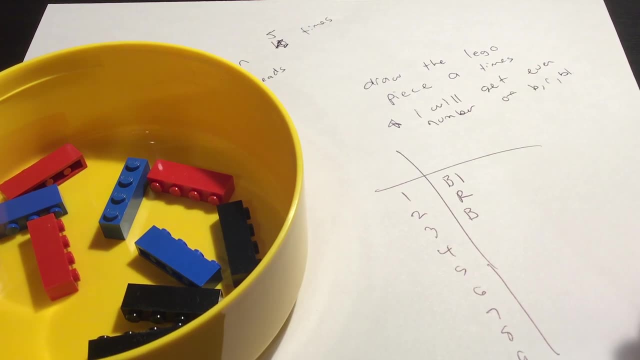 even it could be argued that I would draw, even, I would draw, even, I would draw, even I would draw two blues in a row at some point, at some point- Especially if I said I'm going to do this a thousand times or a million times- right, The chance that I draw blue a couple of times in a 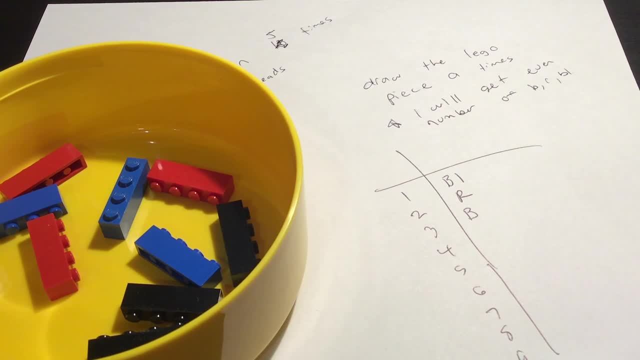 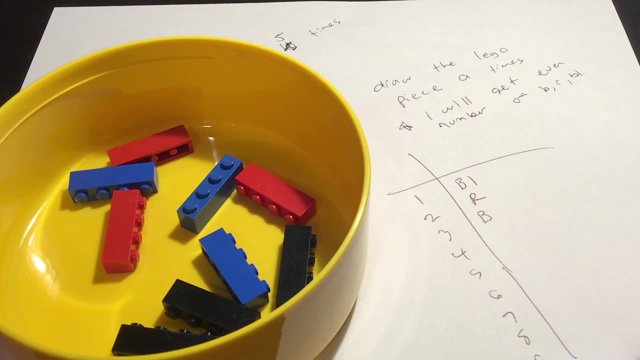 row or red a couple of times in a row. that's going to happen. It's almost certainly going to happen. I'm not going to always get the same order over and over again. one each three tries Mathematically. yeah, sure, That makes sense, But in real life that's not going to happen. Just. 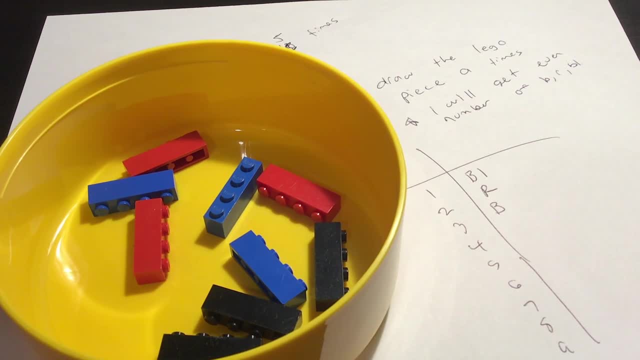 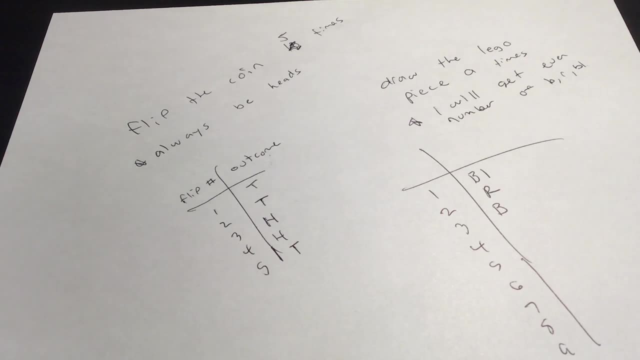 like, if you play Monopoly with your family, do you ever roll doubles? Yeah, Sometimes you roll doubles. right, I might pick two blues in a row. You never really know. okay, And that's kind of the key point to the last thing that we're going to talk about, which is how many times you 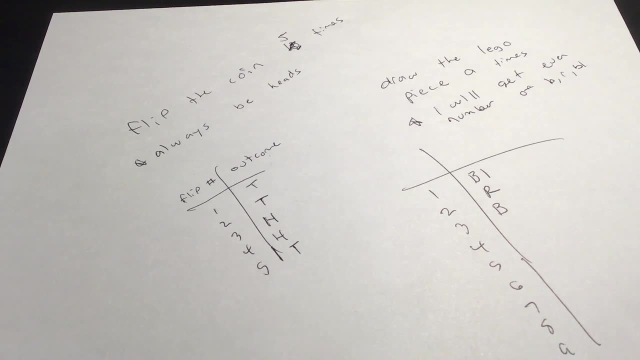 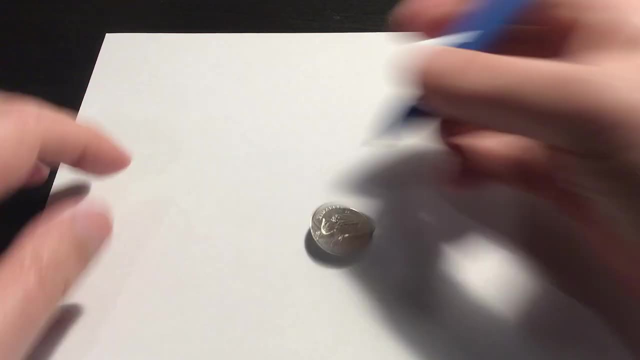 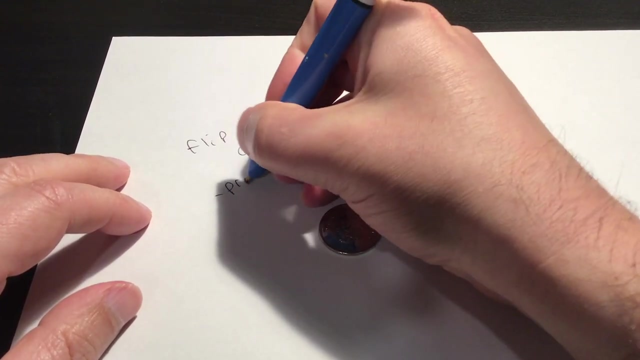 do the experiment? How does that influence what happens in the experiment? So I'm going to flip my page over here. So let's say, my new experiment is: let's go back to the coin. I'm going to flip the coin, Flip the coin And I'm predicting, since I've been learning here. 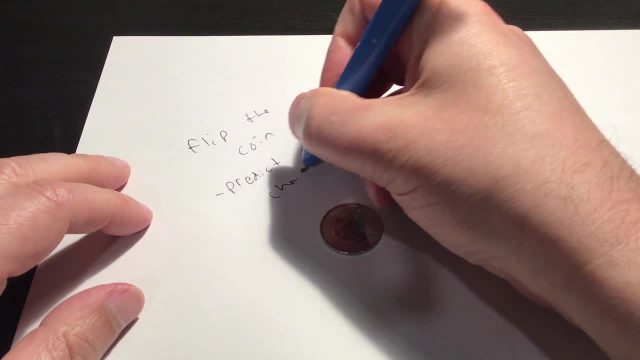 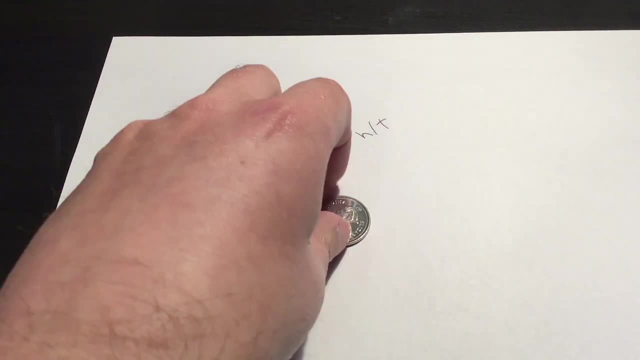 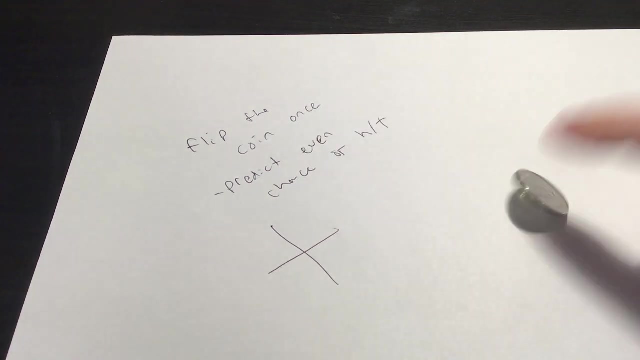 predict even chance of heads or tails. That's my prediction. I'm going to flip the coin once. Here we go. Flip my coin Heads, Flip one Heads. So my conclusion after performing this experiment is that every time you flip a coin you will get heads. What's my proof? 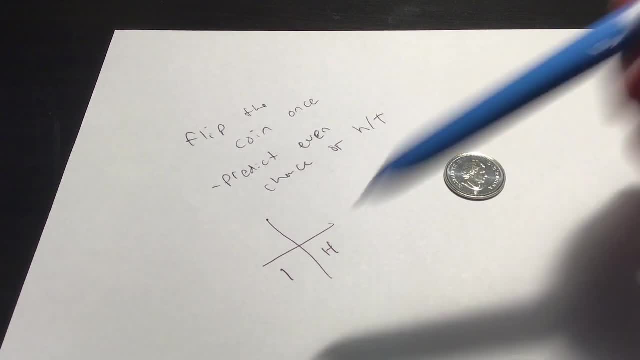 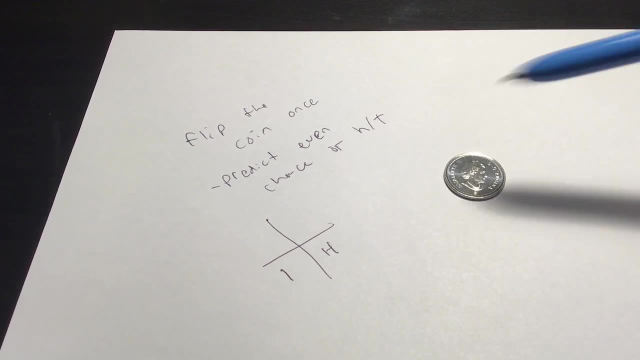 Well, I did an experiment. Here's my proof. I did an experiment, I flipped the coin And every time I flipped it I got heads. I flipped it and it was heads Every time in my experiment. okay, So my proof, therefore, is that when you flip a coin, 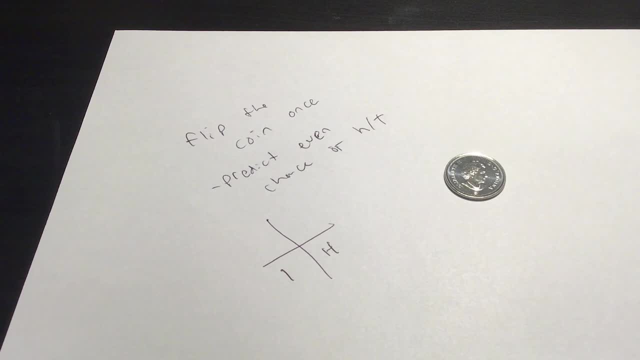 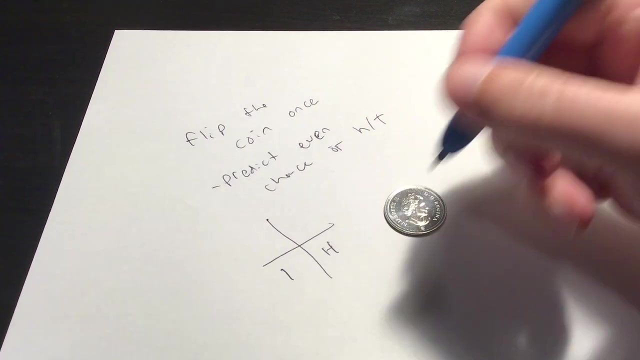 it will be heads. Fair experiment or not fair experiment? Okay, obviously that's not fair, right, That doesn't make any sense. First of all, the coin has two options. So there's no possible way Do an experiment without at least doing it twice. And if I did it twice could I get heads. Let's. 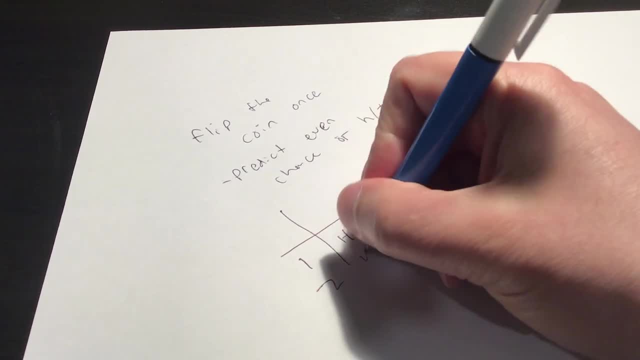 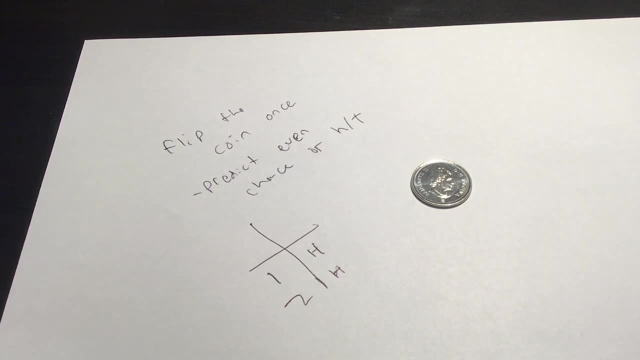 just pretend: Oh, I flipped it. Oh, heads again. Oh, therefore, you know, shut it down. The evidence is complete Every time you flip a coin. it's definitely no, okay, You have to do the experiment more times than just a couple, right? What do you think would happen if, let's say, we got the whole? 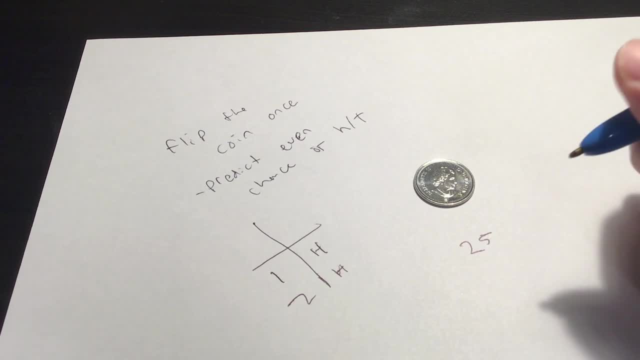 class together. Let's pretend that there's 25 kids in our class. okay, And we each do the experiment where we flip a coin and we only flip it once. So let's pretend that there's 25 kids in our class. 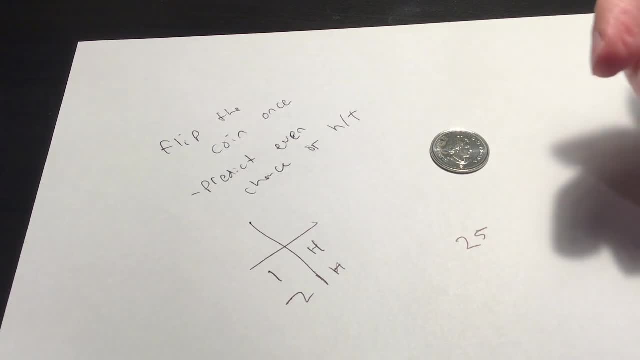 okay, What do you think would happen in the class? Is it possible that all 25 kids would flip heads on their experiment? It's possible. okay, It's not impossible using our probability talk. It is possible, but it is very unlikely. okay, If I flip a coin once, my chance of getting heads is 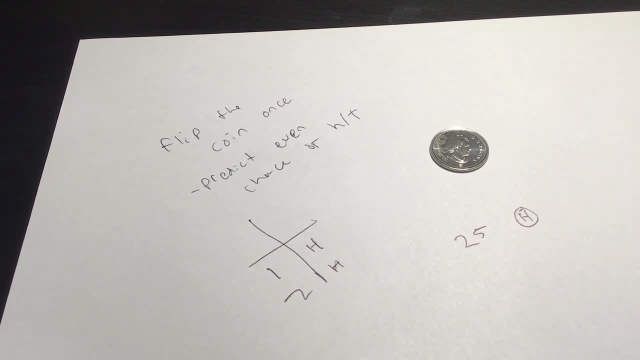 equally likely because there's only two choices: It's heads or tails. So if I flip a coin once and I'm trying to get heads, I got an okay chance, an equal chance of getting that heads. But the more you know times, I add to. 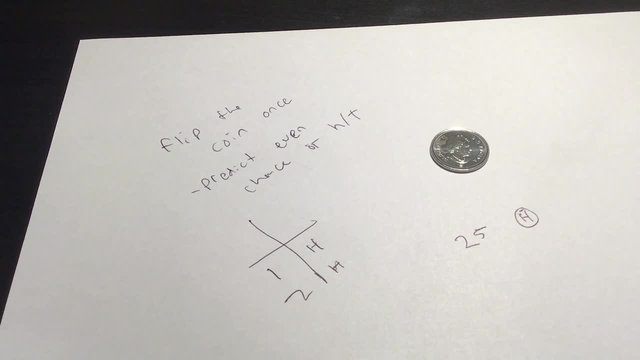 this experiment, the less likely I'm going to get what I want. So if I said I want to have heads every time, that's what I'm trying to prove, because, like I'm some weirdo or whatever and I have 25 kids, flip it. the chance of all of us getting heads is very unlikely, right? We would. 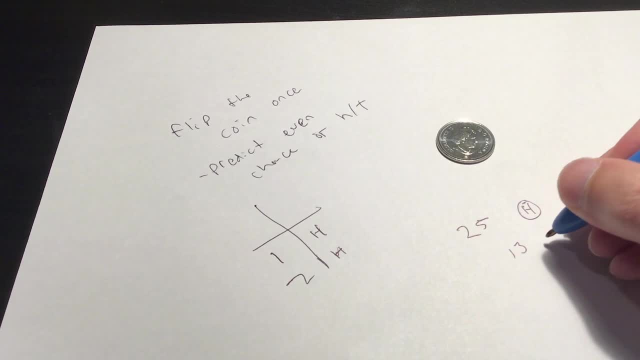 expect to see. you know, 13 kids get something and 12 kids get heads. So if I flip a coin once, kids get the other, It might not work out that way. right, You know we might get, you know. 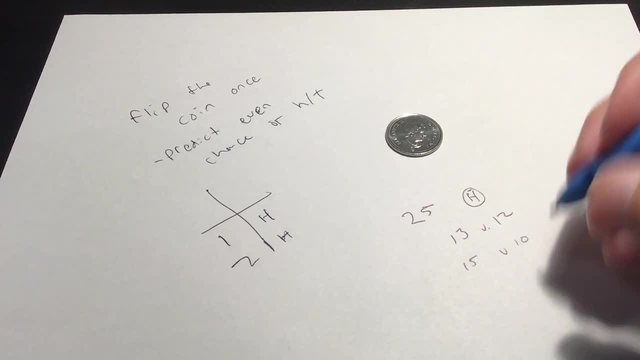 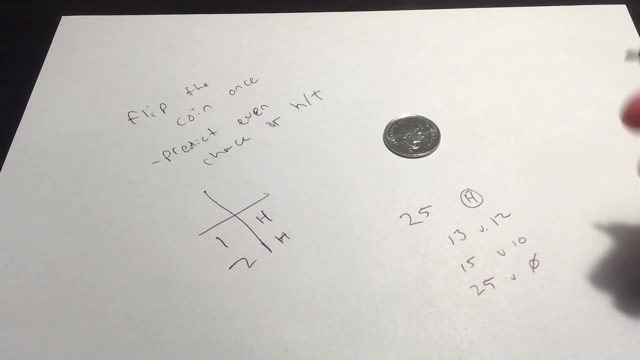 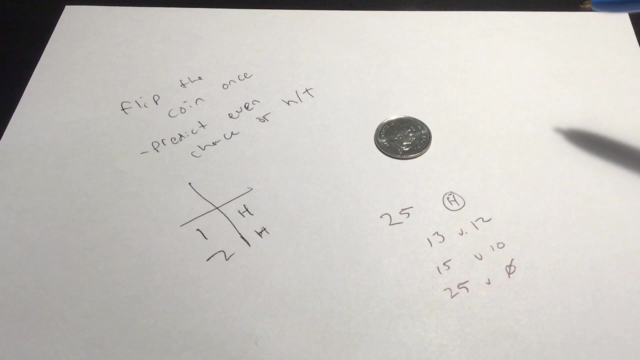 15 versus 10 or something like that, but we're probably not very unlikely that we're going to get 25 one way and zero the other way. Could happen, right, Could happen, but it's very unlikely. We're more likely to see something that is closer, okay. So that's sort of the second point of these. 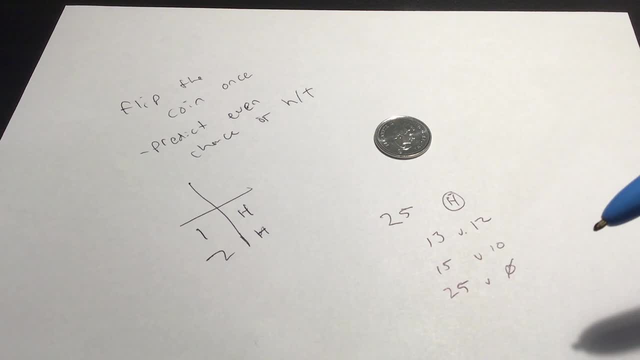 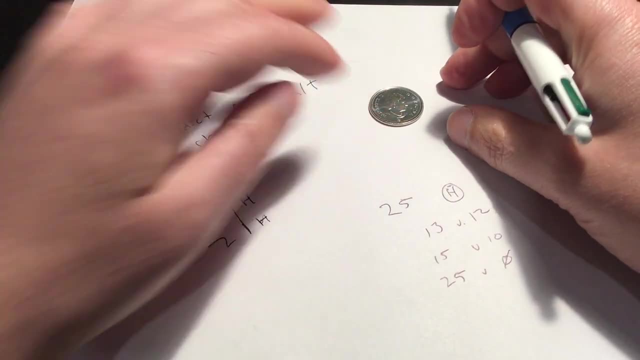 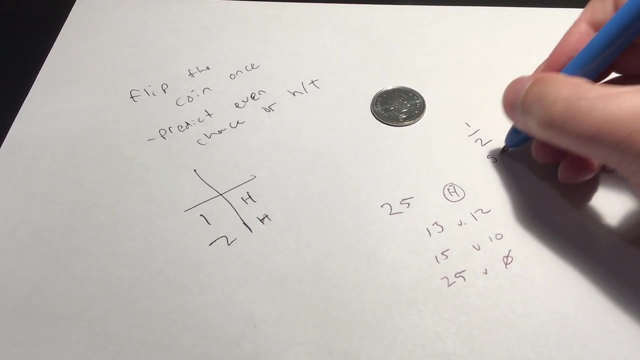 experiments is that the more times you repeat the experiment, the more likely you will see. okay, so i expect if i flip a coin i will see heads or tails, and if i flip it a million times i would expect to see about half the time. so 500 000 times heads and 500 000 times tail, that's what. 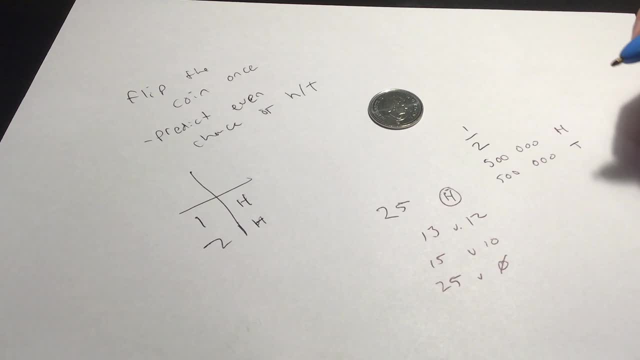 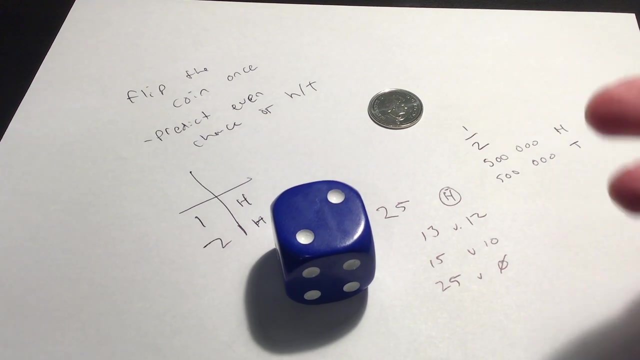 i would expect to see. now, it might not be perfect, you know, but the more times you do the experiment, the more times you will, or the more likely you are to get to the sort of mathematical idea. right, if i roll dice six times, i might not get a one once. a two once is three, right, i mean. 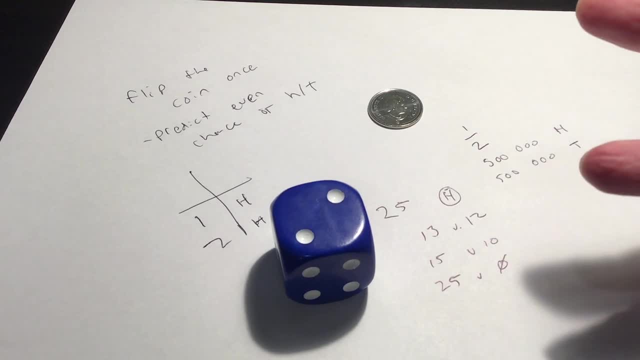 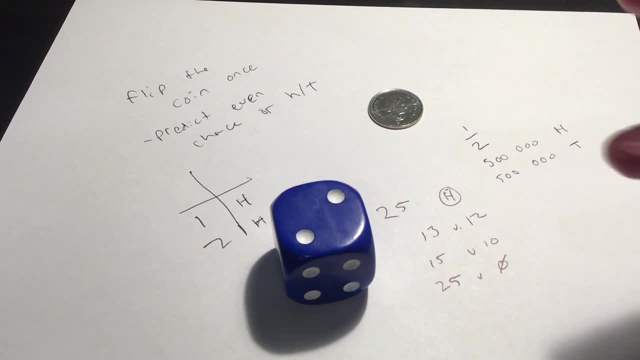 a million times for each number, maybe not perfect, but pretty close. if i do the experiment six million times, i would expect to see somewhere around a million times. did it six million times, I definitely would not expect to see three come up four million times. I. 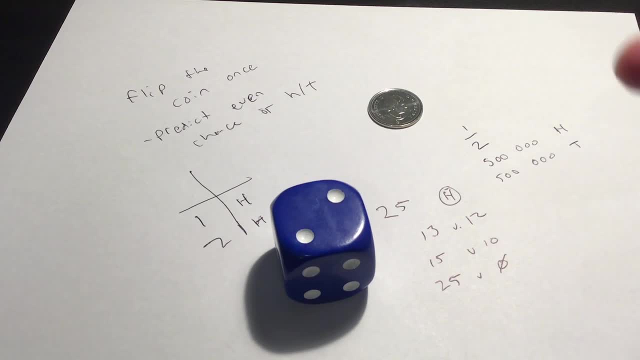 mean, that is, you know the math behind that. it makes it almost impossible- Not quite, but almost impossible, All right. So that's sort of the two things I wanted to bring about today: The idea that one that you can create an experiment, a probability experiment, where you, you know use. 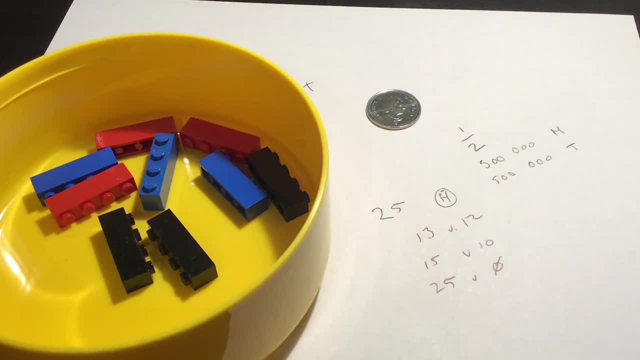 dice or coins or whatever you have around the house, to think of the experiment and then predict what you think will happen. Okay, And we call that sort of like a theoretical probability. So it's it's the idea that what we think should happen And we can use math to come up with that. 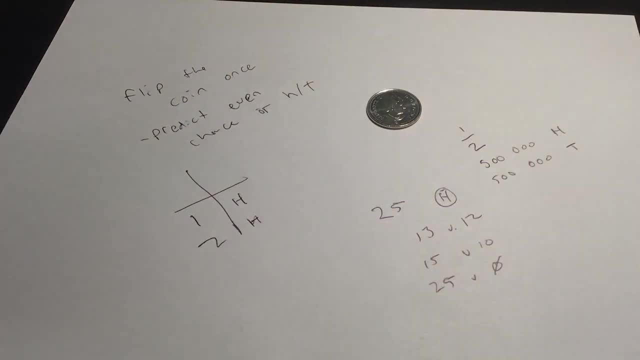 And you will do that in later grades. Then you conduct the experiment. Okay, And just to keep it interesting, just do the experiment once, or just do it twice. Try to just do it a few times and then bump up, bump up those numbers. Okay, So like if you're flipping a coin, try just flipping. 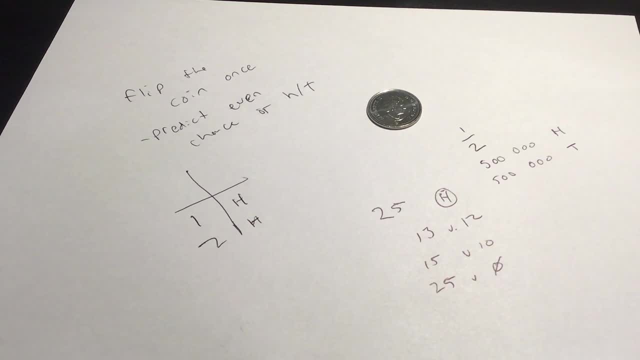 a coin twice and seeing what happens. Maybe you get head, heads, maybe you get tails, tails, maybe you get a mix, Um, but then try it 20 times and keep track and see if you get closer to your prediction. Okay, Um, so there you go. There's a little bit on probability- Probability by the 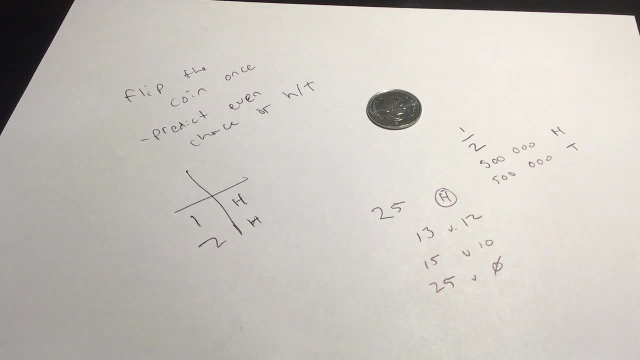 way is one of those things I I feel like, if you speak to adults, um, unless they're sort of like math teachers or somebody who's really into math, they don't really understand probability. And I have proof of this, by the way, that people don't understand probability. My proof is people play. 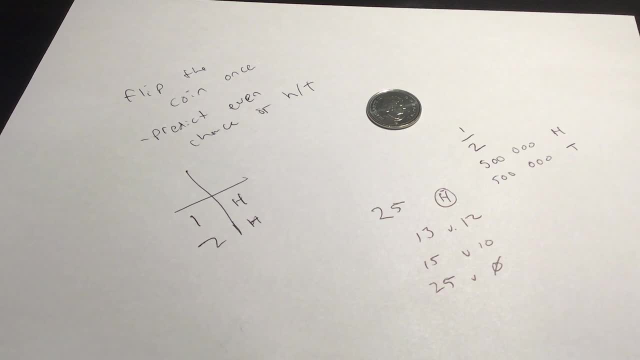 the lottery, People go to casinos. Okay, These things make a lot of money, And the reason why these things make a lot of money is because the people who run those things do understand the math, Okay, And they make games or lotteries that make them money They don't make. 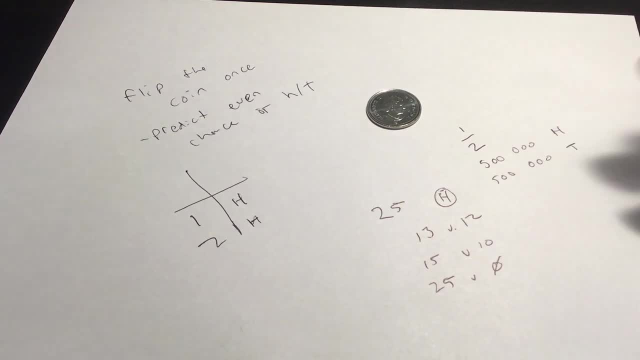 a game where the probability is in your favor, because then they wouldn't make money. Okay, They make games where the probability is that they will make money. Could they make some? you know casino game, where people are pulling those handles and everybody wins. It could happen. 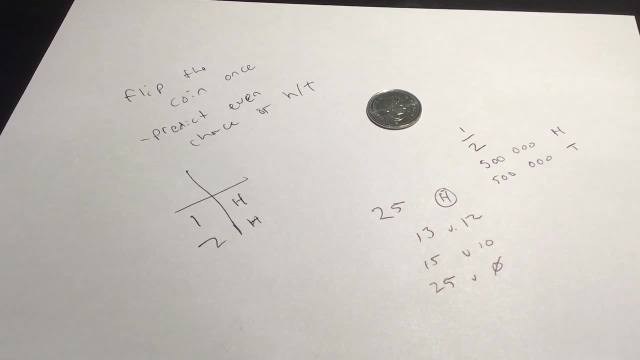 but the probability is very low. Okay, They make games where the probability of them winning is very high and that's why they make so much money. Okay, So there's sort of my my own little theory and my evidence for it. Okay.